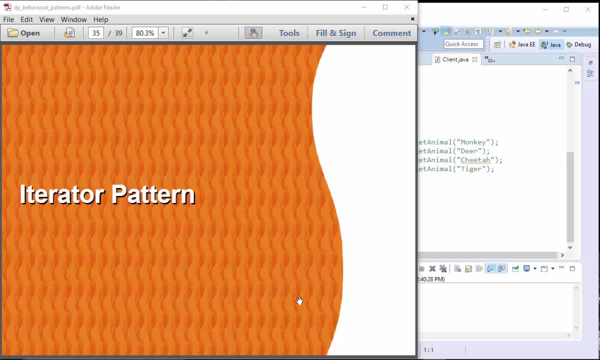 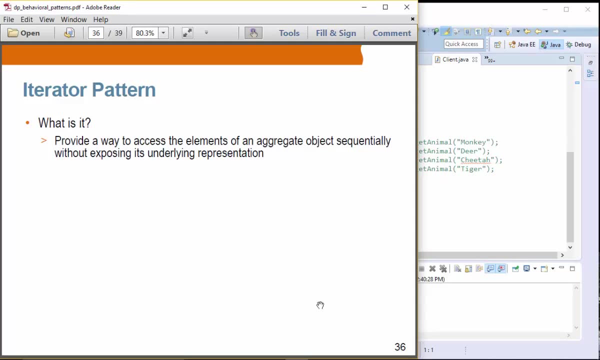 The last pattern we are going to look into is iterator pattern, The last pattern in behavioral pattern. So what is iterator pattern? It provides a way to access the elements of aggregate object sequentially without exposing its underlying representation. So if you happen to have a case where you have some internal aggregate of some object and you do want to hide that internal aggregate structure, instead you want the client to be able to access the object in sequential order. that's when you want to use iterator pattern. 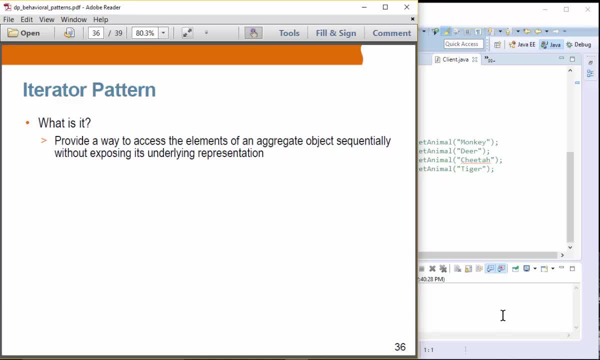 And Java already provides iterator right, So we are going to just simulate it. So Java iterator is important, In fact, using the iterator pattern. So we have iterator interface. It represents abstraction defining iterator. I should actually rewrite this statement. Then we have a concrete iterator which basically implements the iterator Basically. you know isNext, getNext and things like that. 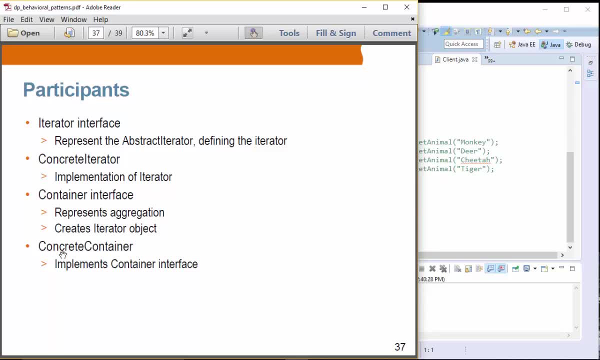 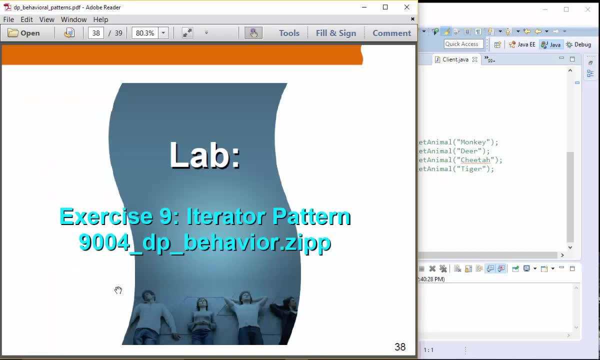 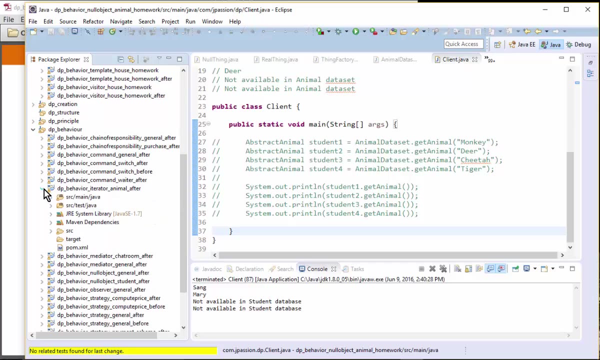 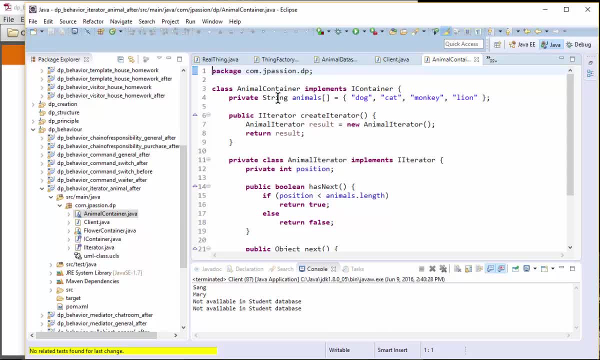 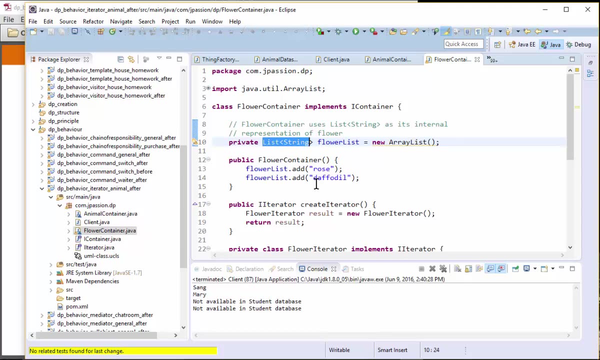 So one is admult container and this one is actually maintaining animals in a form of array. So this is internal aggregator, So this is an array representation, It's using array. And then we have a flower container. Flower container is using list of string as internal representation. 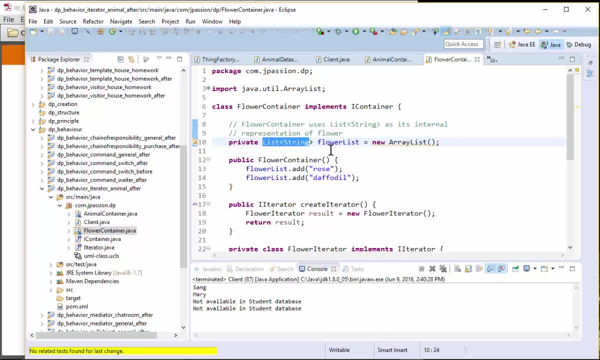 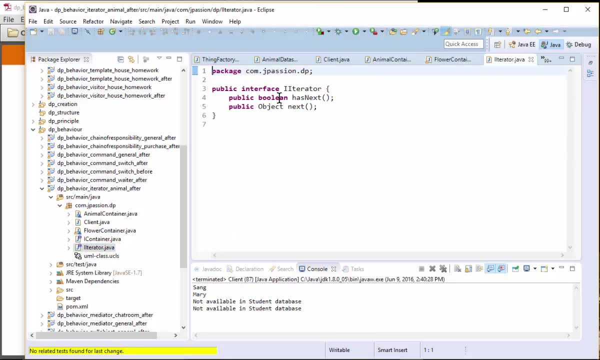 Now what you want to do is: we want to provide, you want to hide this internal representation from the user. So user will just use iterator interface. So iterator interface is basically hasNext method and the Next method. Okay, And then we have actual iterator. 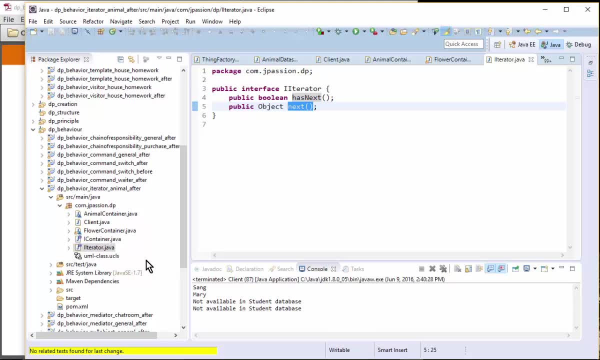 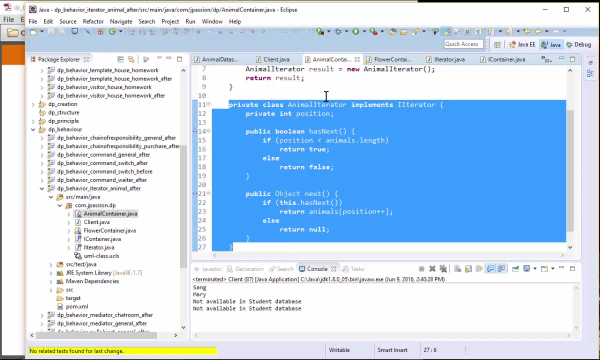 And then we have the actual, the I container. the I container will actually create the actual I iterator object. And then we have the animal container contains this. you know, in this case we actually have the inner class, called the animal iterator, which implements this iterator. 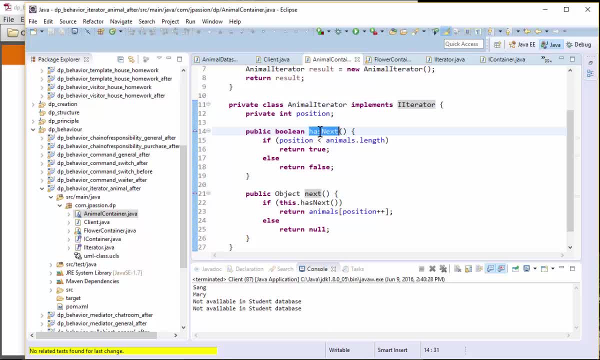 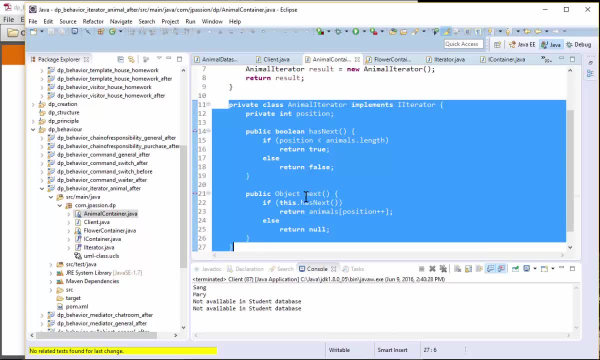 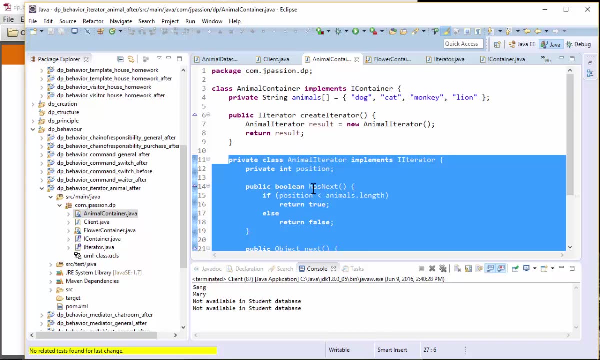 And basically this animal iterator. This iterator will provide the implementation of hasNext and Next. Okay, You know, we actually make this one as internal class because this is used only in the context of this internal representation. Okay, I mean, you can certainly take this out if you want to, but because the it access. 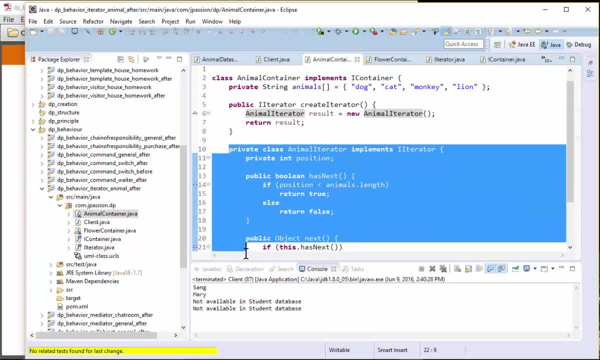 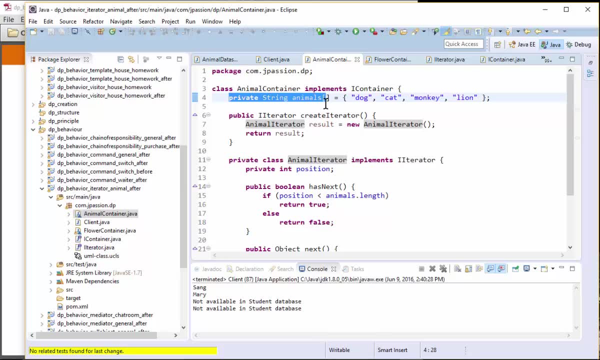 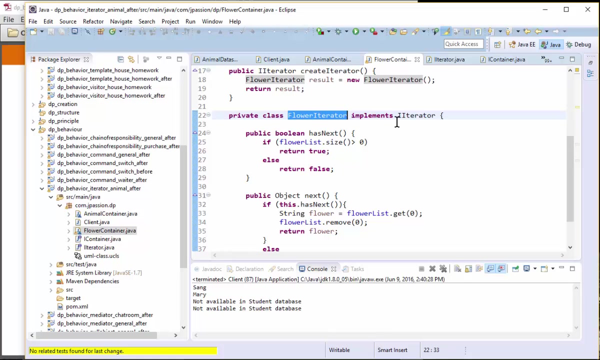 yeah, in fact, you know what this is actually internal class because it has to access the private, the attribute of the apparent class. Okay, So in this case it has to be internal class, the inline class like this, And the flower container again provides the flower iterator object, the class implementing. 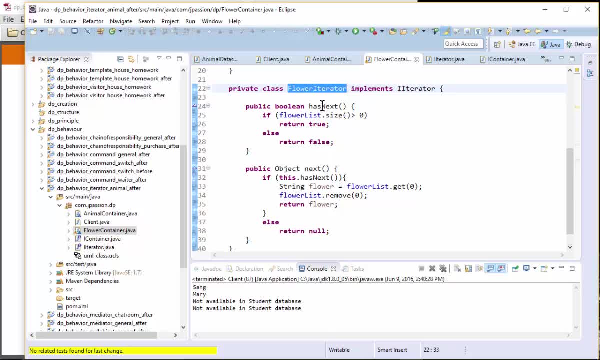 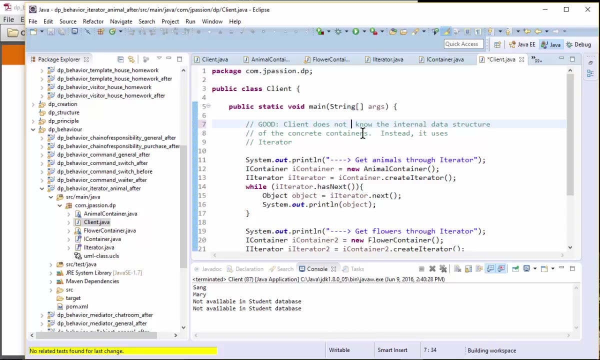 iterator And basically, you know it does implement hasNext and Next the method implementation. Okay, So as far as the client is concerned, the client is concerned, it, you know this good part, Okay, Client does not need to know. I should say need to know. client does not need to know. 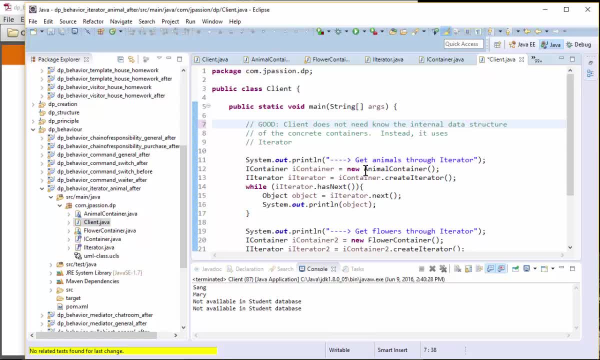 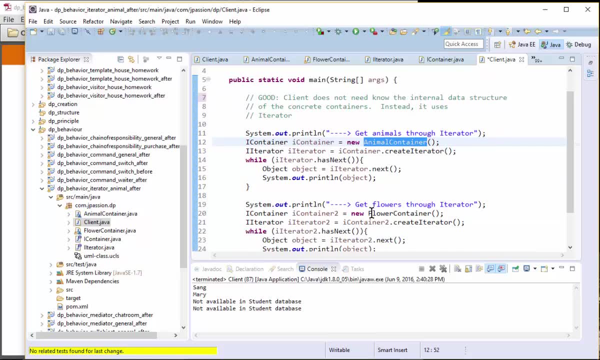 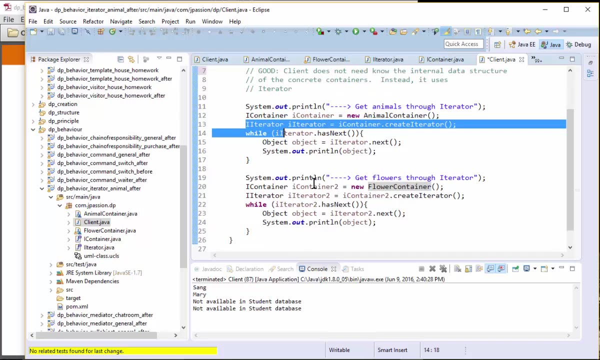 the internal data structure of the containers. It doesn't know how animals are in fact represented inside the animal container. It doesn't have to know how flower is actually represented internally. right, It just used the iterator. Okay, So you know, basically, if I run this code. 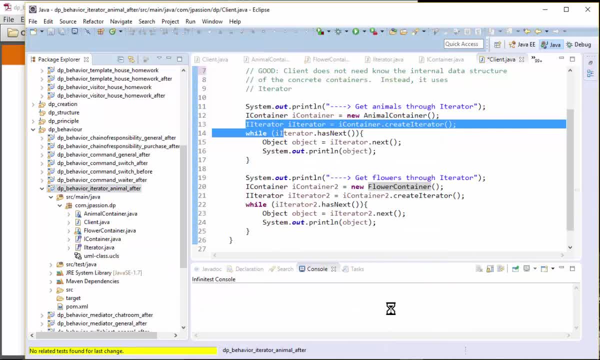 Okay So it's just accessing animals and flowers, So this code does not need to be changed, regardless of the internal aggregate representation of animal container and flower container. Okay, So the it actually provides some kind of abstract way of accessing elements in that.